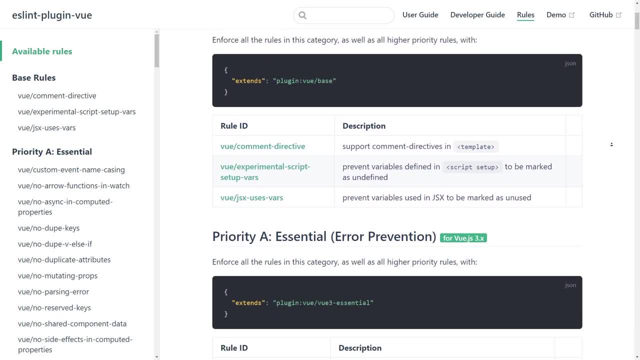 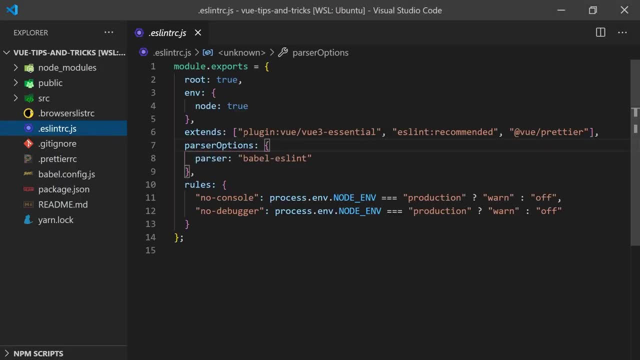 You can automate some of this by using the Vue ES Lint plugin, which comes pre-configured. when creating a Vue app, using the CLI tool, You can go into the ES Lint settings and change it from Vue 3, Essential, to Vue 3, Strongly Recommended for an improvement in code readability and dev experience. 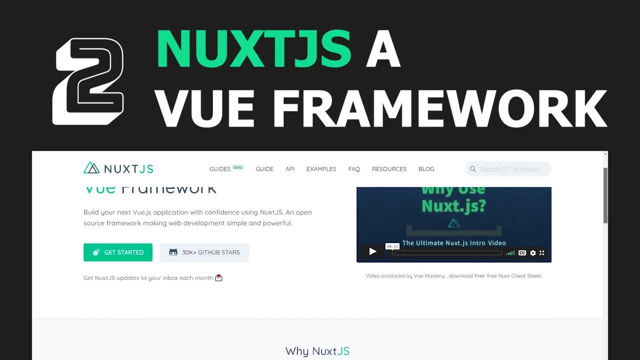 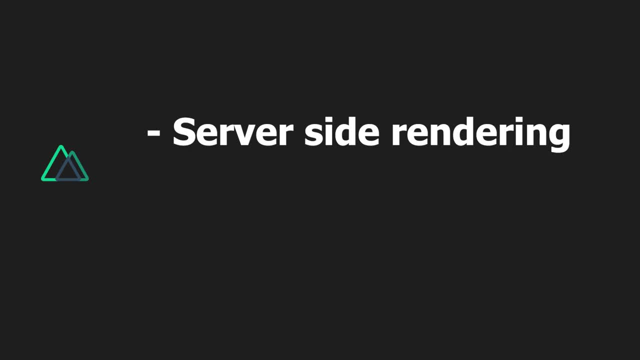 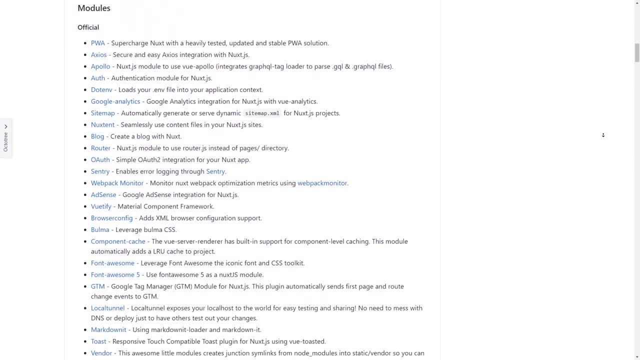 You should also consider using Nuxjs, once it's available for Vue 3.. If you plan to build a production-ready Vue application, it can solve many of the problems you face, such as server-side rendering and dynamic routing. It also provides an ecosystem of plugins which you can use to build your application faster. 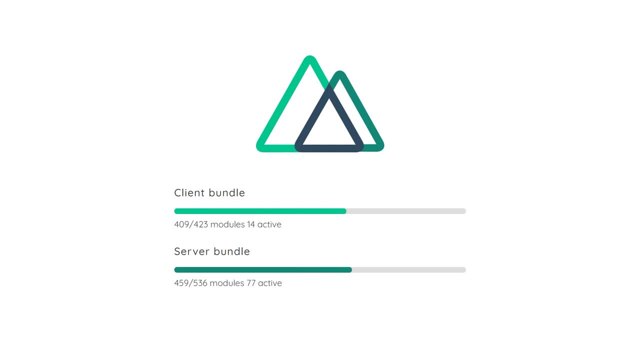 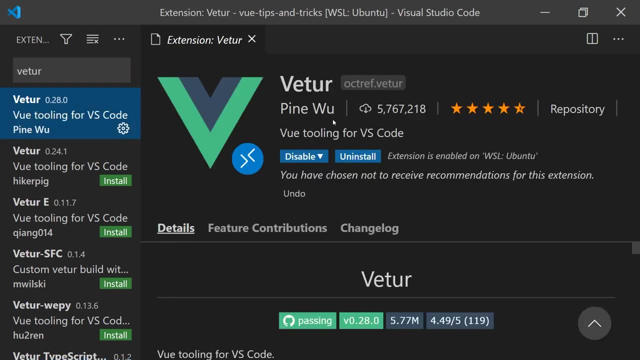 Most importantly, it comes with a nice loading screen, so you have something to look at when your application is compiling. Now we can head over to Visual Studio Code, where you should already have VueChair installed. You can make this plugin even more useful by enabling the experimental. 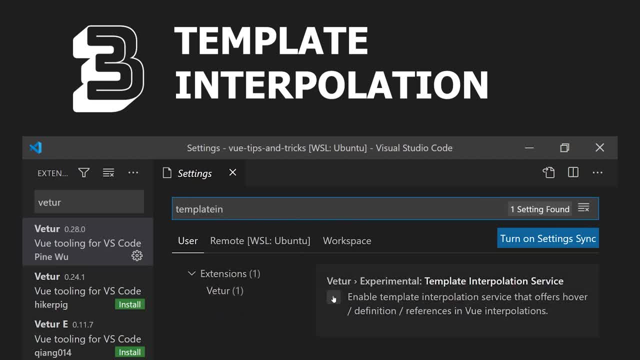 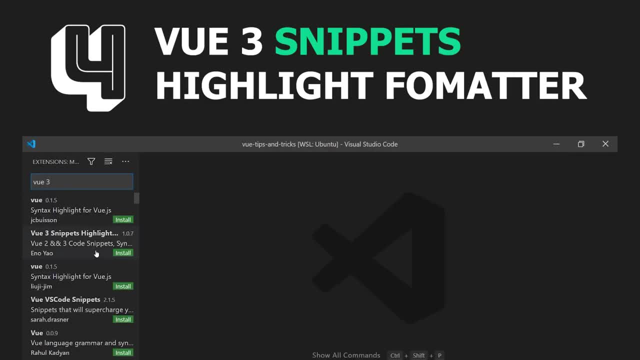 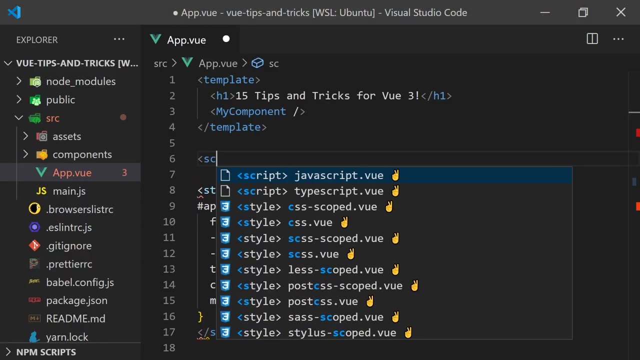 template interpolation service, which adds even more auto-completion and type lookups in the Vue component template. Additionally, I also recommend installing Vue 3 Snippets Highlight Formatter. This will give you shortcuts for increasing your productivity when coding in Vue 3 or Vue 2.. 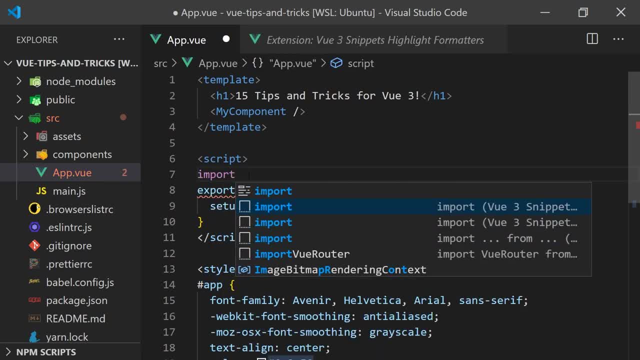 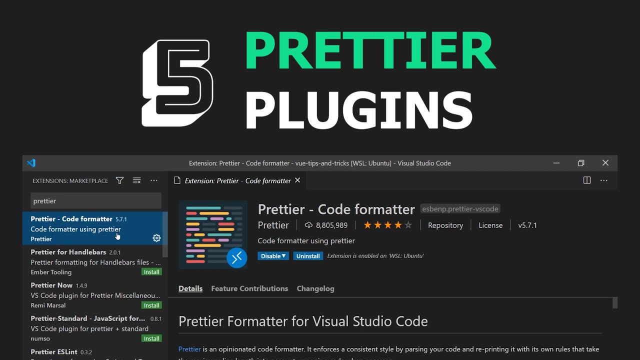 We can now use shortcuts to quickly import functions from Vue and type out boilerplate code required for creating components with just a few keystrokes. And for the last extension, we should also grab Prettier, which will automate formatting your code. This is a huge time-saver and you'll notice I use it in all of my applications. 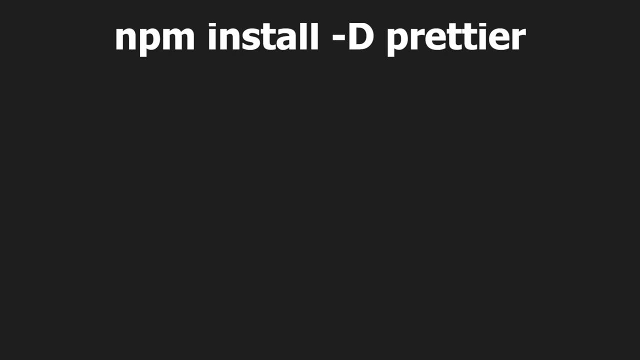 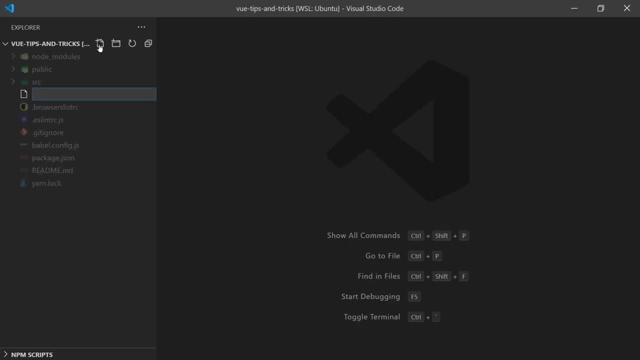 You can install the package library using MPM, Install Prettier, or have it come pre-configured with your Vue app by enabling it in the CLI tool. Now you're able to create a Prettier RC file that describes how the code should be formatted. 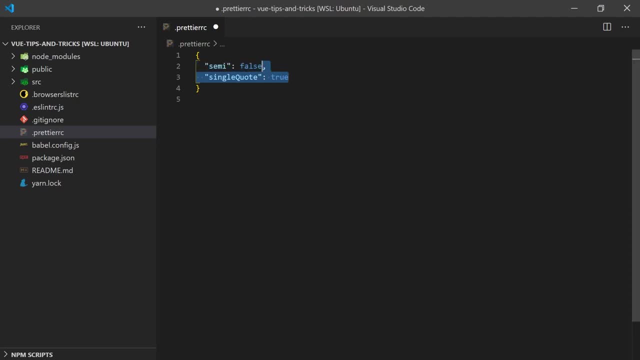 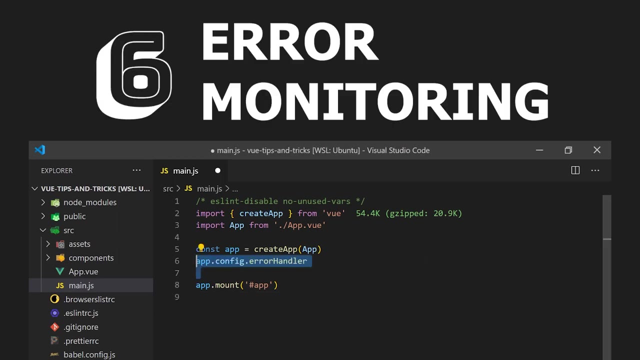 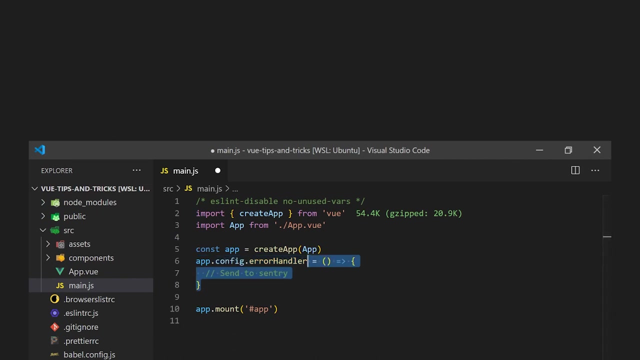 Personally, I like to disable semicolons, use single quotations and remove any trailing commas. Using the extensions we just installed, we can quickly configure our Vue app to monitor errors. Error monitoring is extremely important in production and we can use the ErrorHandler function to send errors to services like Sentry and Bugsnap for tracking. 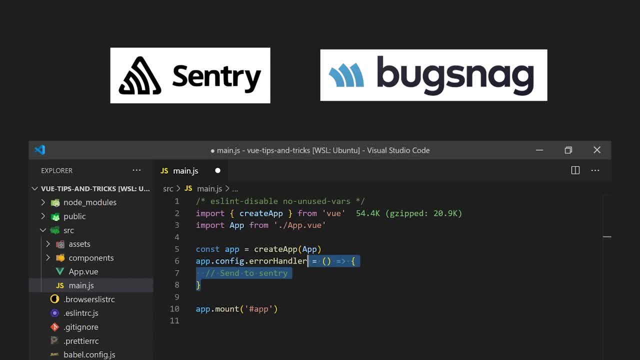 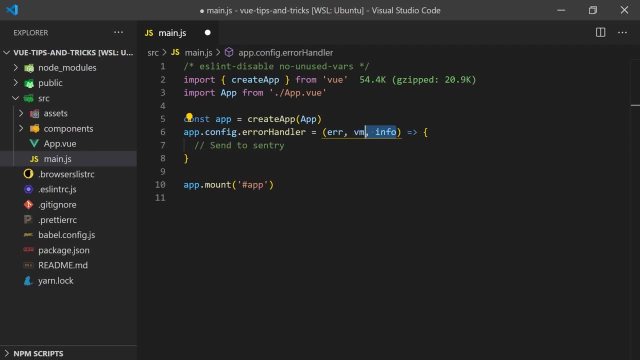 This function gets called whenever an error is thrown inside your Vue application and gets called with three arguments: the error trace, the Vue component and Vue-specific information, such as lifecycle hooks or events that caused the error. You could also add a function to: 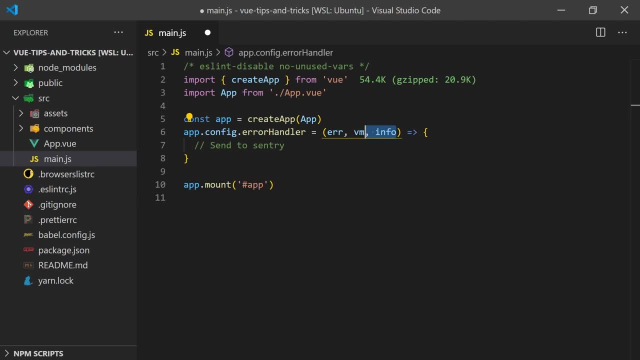 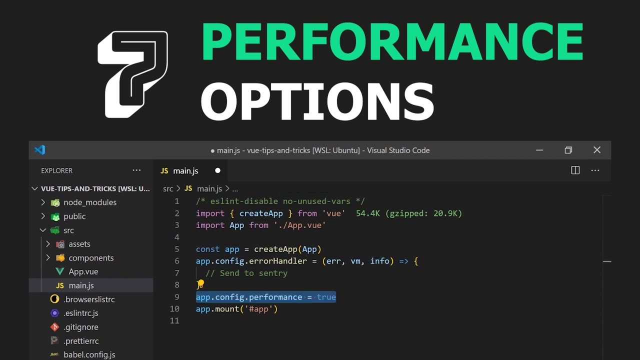 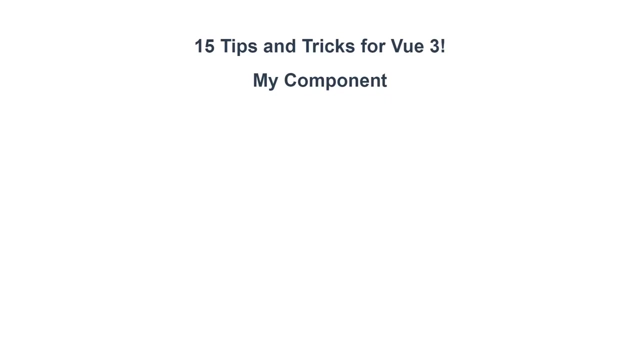 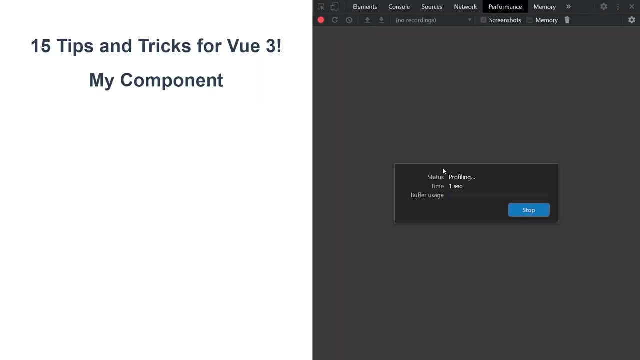 any of your components called ErrorCaptured, which will also be called when any descendant components throw an error. That's extremely useful, but we should also enable performance options in development mode to get more information when debugging. We can view performance information about our components' mounted and render times by going to the DevTools, clicking the Performance tab and then recording an interval we'd like to inspect. 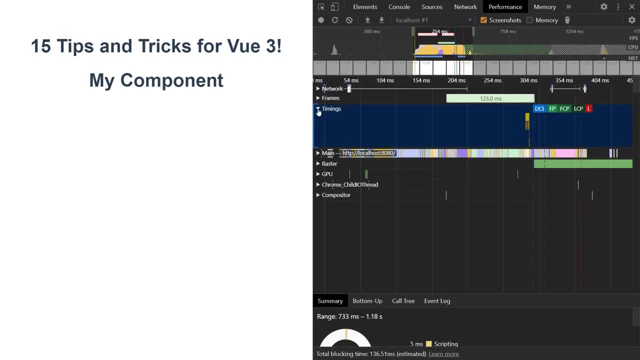 In our example- I'll just refresh the screen Now- going under the Timing section, we can see that the performance is set to 0.. In the Timing section we can see information showing the load times for each Vue component. I'm glad we've got our tools and app set up, but now we should start looking at creating some components. 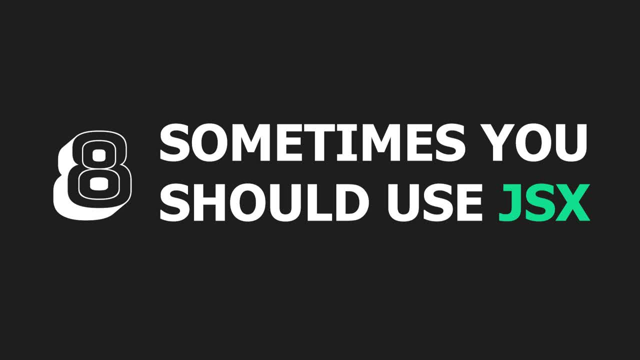 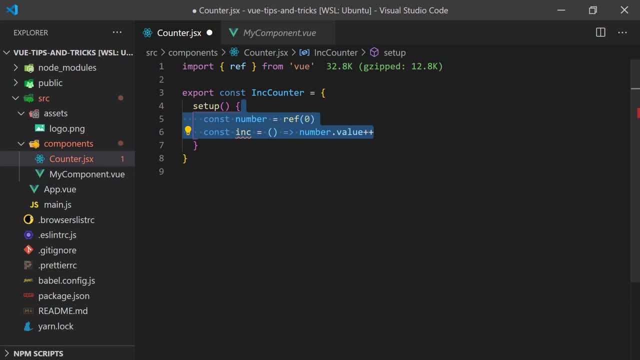 Don't be afraid to use JSX, as you can create small, reusable utility components instead of having to create a new file for each one. For example, we can create two simple increment and decrement counter buttons, which will apply the operation whenever the button is clicked. 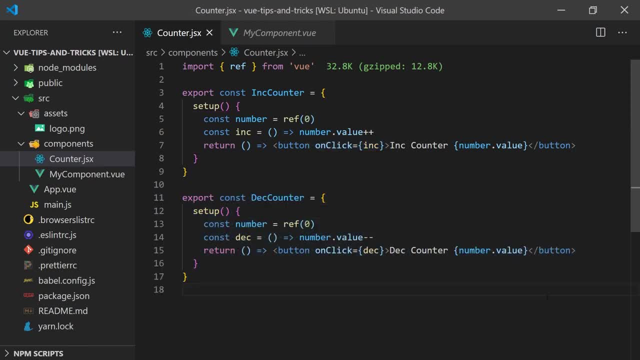 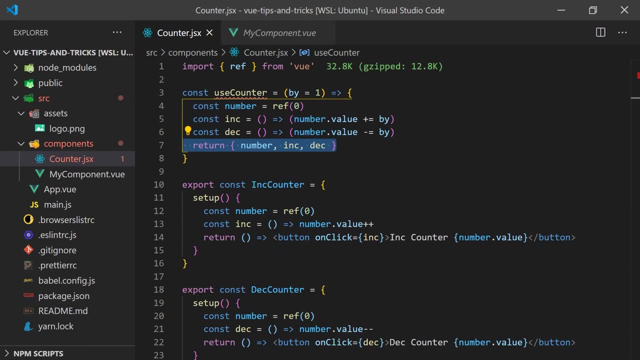 Similarly, The new Composition API makes it really easy to abstract away common utility functions that may be useful across multiple projects. We can demonstrate this in our example by creating a useCounter function that will accept a value to increment and decrement by and return these functions, along with the number value itself. 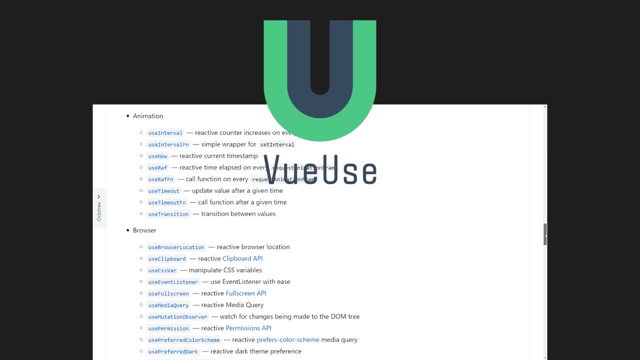 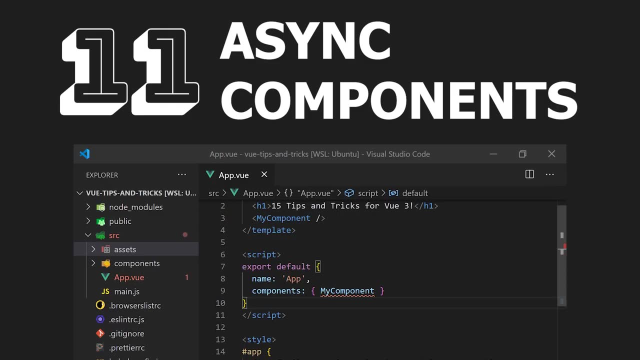 I suggest you also take a look at a library like Vue use, which comes with a whole bunch of utility functions. The link can be found in the description below. When we import our previously created components, we can use asyncComponent to improve loading times. 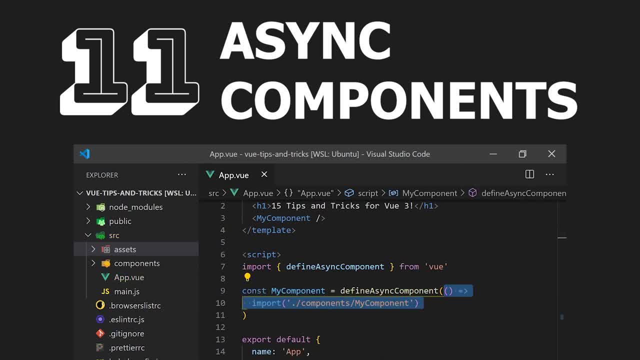 Using the import statement, we are able to create a separate JavaScript file that will be requested when the component is required. This saves your users from loading components that they may never need. If you'd like to learn more, you can check out my other video, where I go over this topic in more detail. 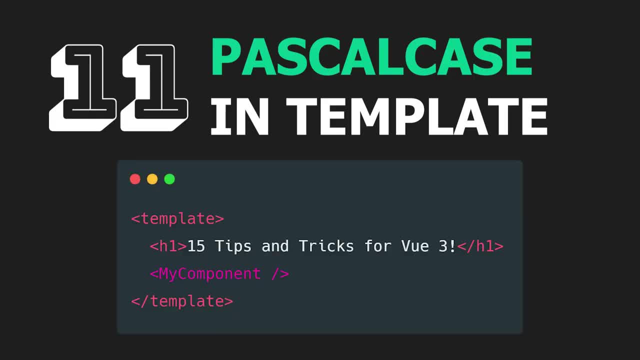 When working with these components in our template, we should always use Pascal's case. This makes it easy to differentiate between HTML and Vue And, depending on the extensions you have installed, it can also give them a different highlighted color, making it even more clear.